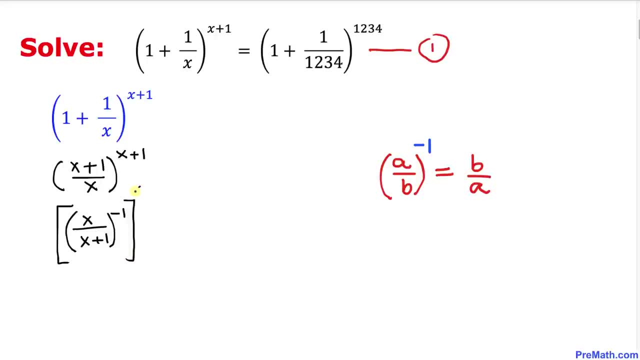 and then put another power, x plus 1, and now we can write x plus 1 divided by x and everything is raised to the power. x plus 1 can see that we have these two nested exponents. and now we are going to use this power rule. 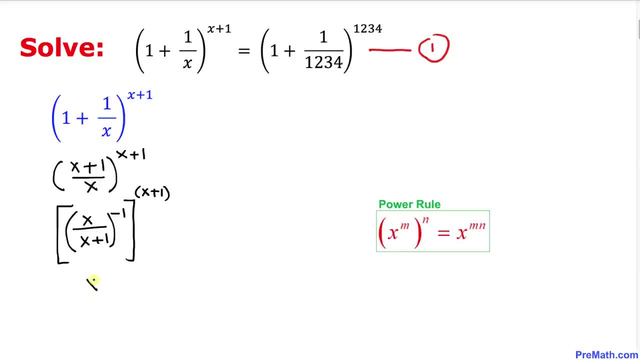 so therefore, we can write this one as x divided by x plus 1, and then power negative 1 times x plus 1. and now let's focus on this base: x divided by x plus 1. I have just copied it down over here, and this could be written as: in terms of this notation: 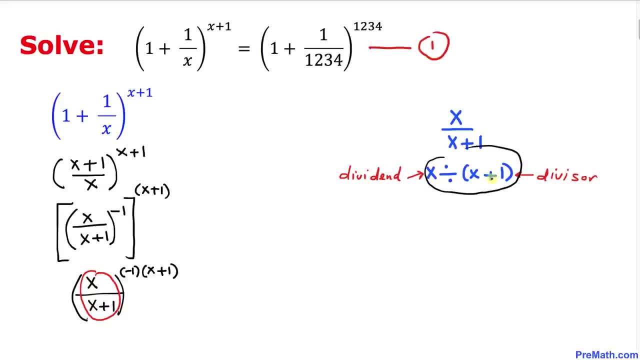 as well, where x is our dividend and x plus 1 is our divisor. and now let's go ahead and perform this simple long division. so we are going to multiply this part by 1, so we can write this: one, x plus 1. let's go ahead and change the sign. this become negative, negative. 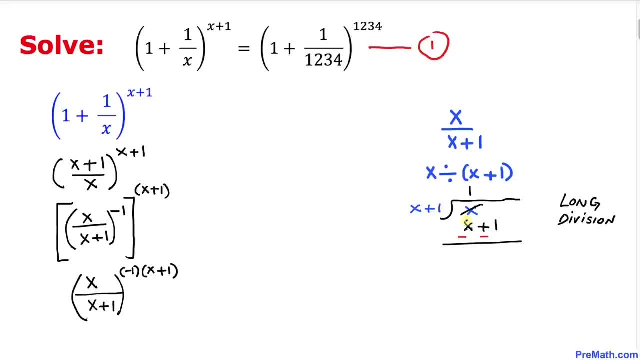 so this could be written as this: positive x and negative x. this is gone, so we ended up with just simply negative 1, so this whole thing could be written as 1 plus this negative 1 divided by this divisor x plus 1, and we can further write it as 1 plus 1 over. I can put this negative. 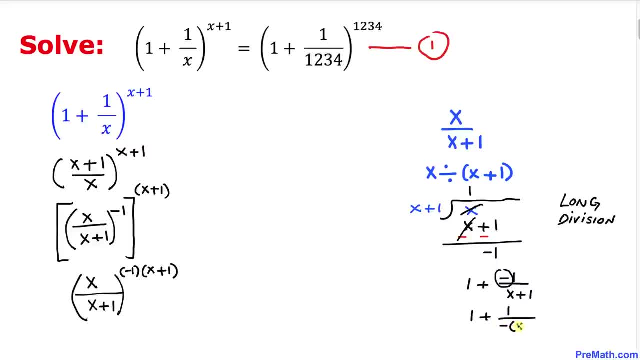 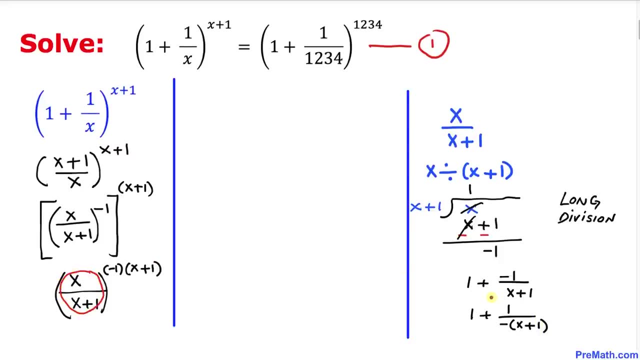 in the denominator by just putting negative x plus 1, and now I can replace this base by this part. all right, so we can write it as 1 plus 1 over negative x plus 1 and then whole power. this thing could be written as simply.